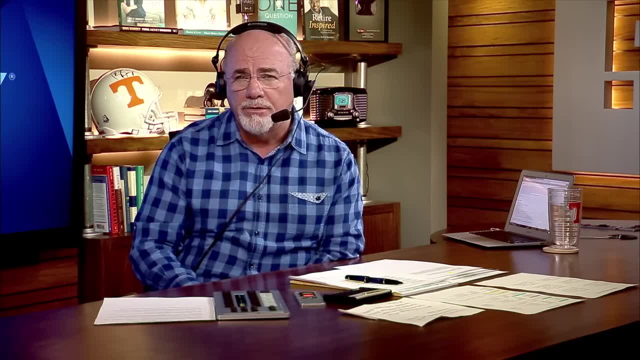 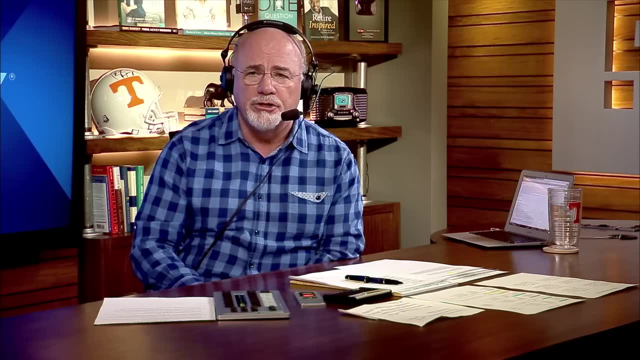 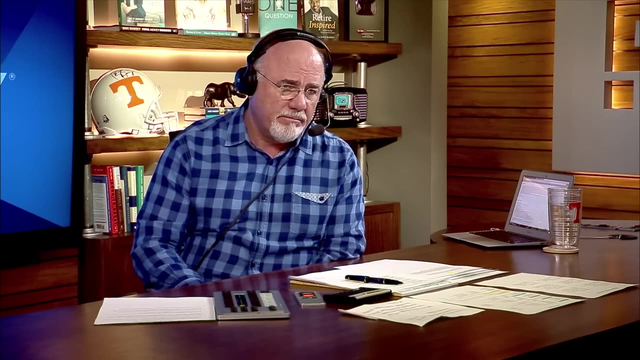 the investment waves like we've had in the stock market in the last couple of weeks. Right, And giving the power of generosity to completely change you. when you learn to give as the natural rhythm of your life, it changes everything. So giving, saving and spending. 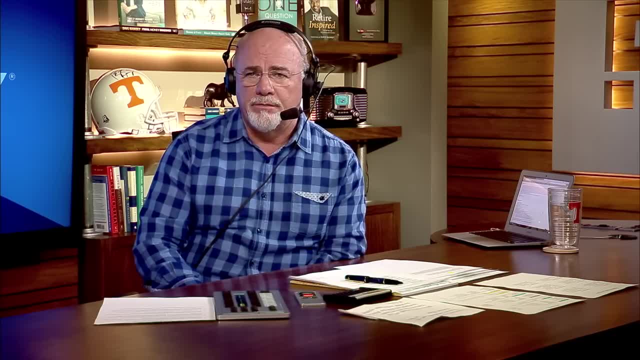 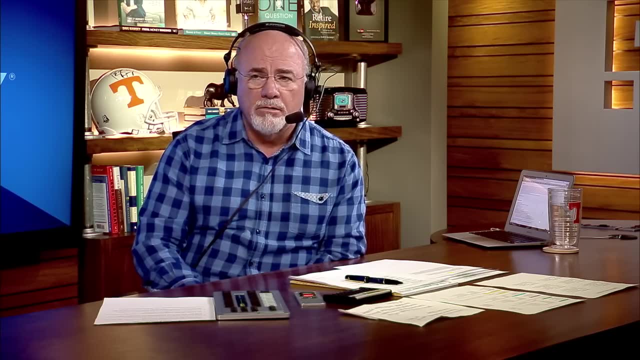 Everyone has at least one of those that they struggle with. Mine is saving. I'm a spender. No trouble for me to enjoy money. It's also no trouble for me to give money A lot of spenders. it's easy for them to be generous because the release of money 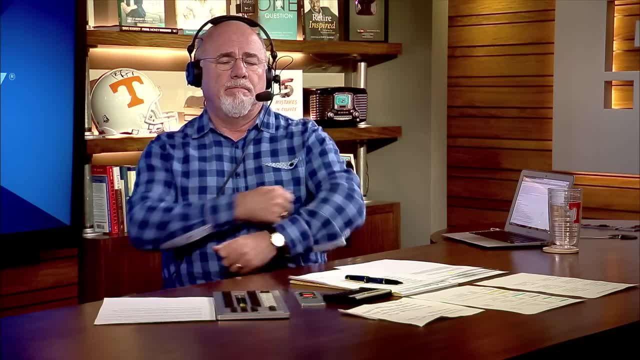 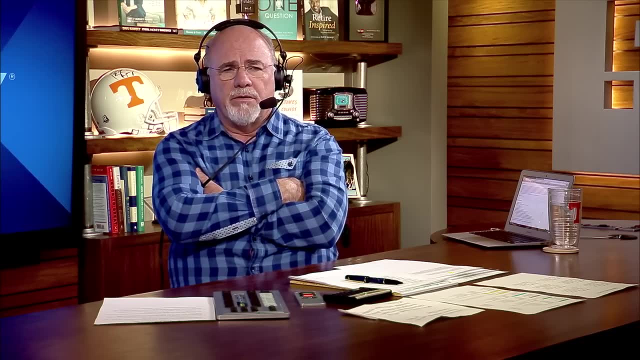 doesn't bother us as much as it does a saver And if and so, but I'm weak at saving and that's why God makes me teach this every day. I'm no longer weak at saving, but it wasn't my natural default. I had to intellectually decide. 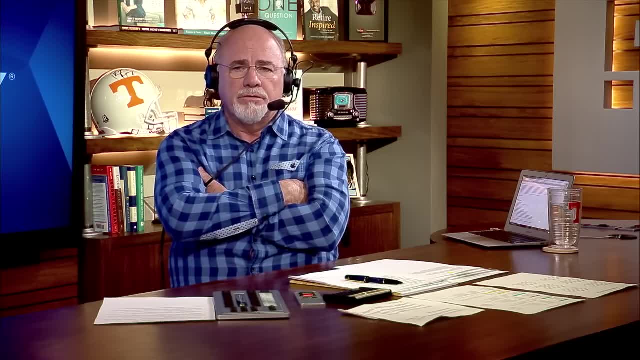 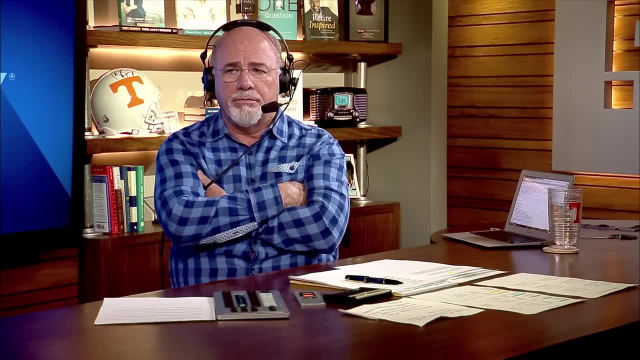 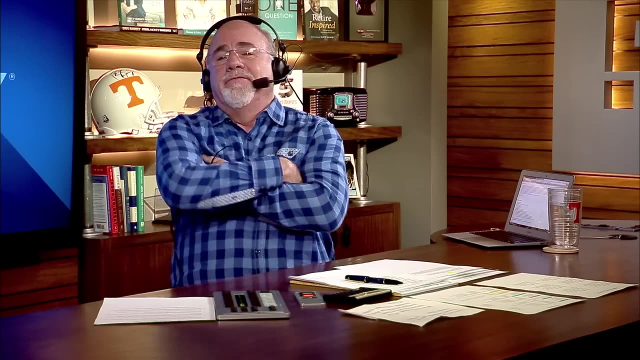 to have an act of my will to save and invest, And really what drove me to do that, as a spender giver, is that I would have more to spend and give. if I built more wealth, I can spend more and give more, And that's my only reason for saving. It's not because I just love saving. 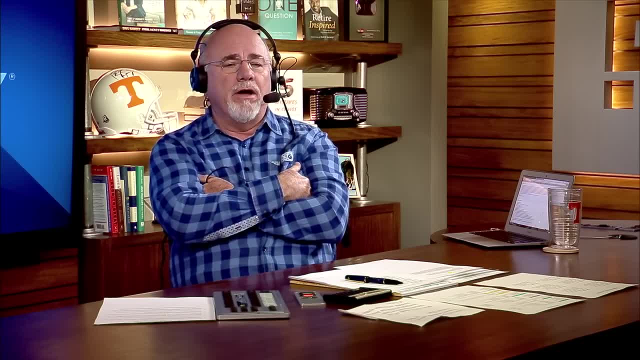 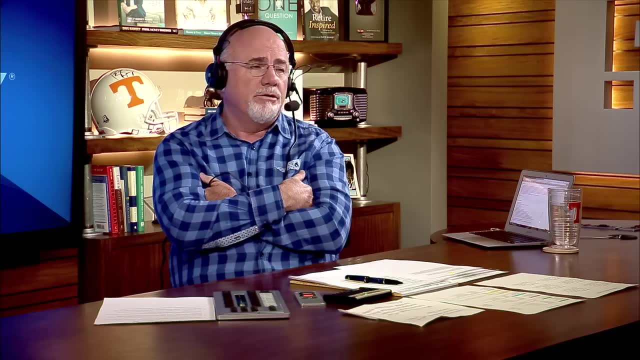 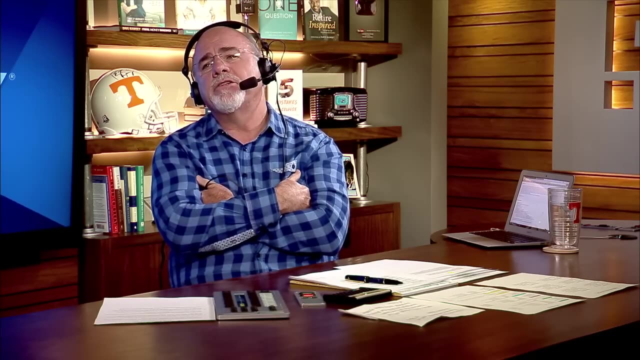 money. I still don't to this day. It's not So. you're on the other side of this, Ricky. is what we're saying? You don't enjoy spending. We don't know about giving. You didn't address that in your thing. Sometimes I can get spenders or savers like this to turn loose of their money. 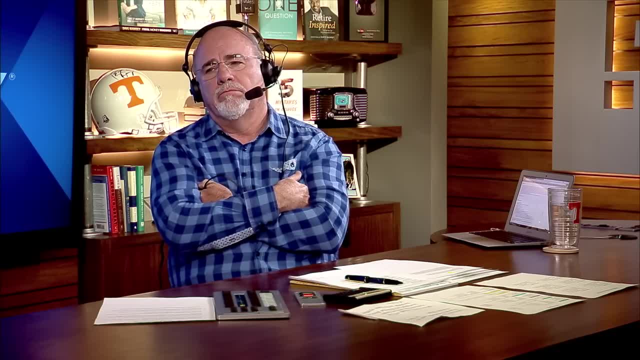 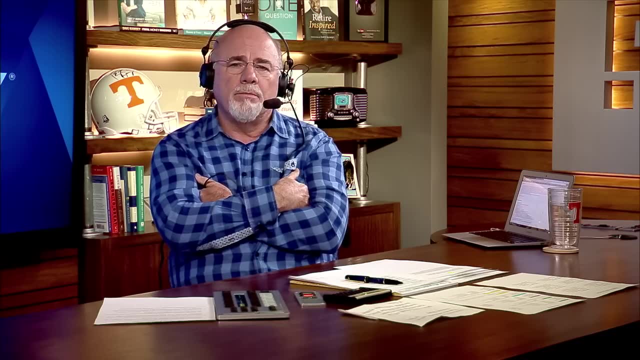 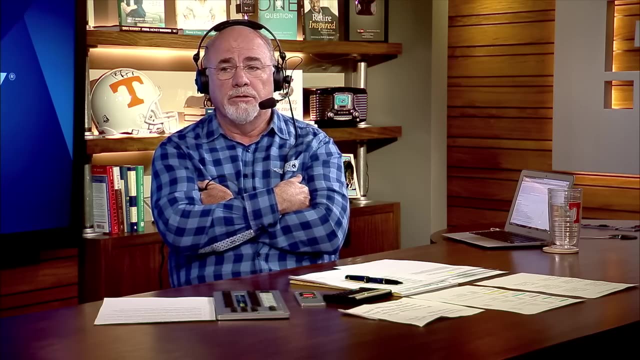 first by increasing their giving And then that kind of gives them permission to also enjoy the money themselves. But it would be a shame to save and work, Not enjoy some of your money, And one of the things you should enjoy is a reliable vehicle. 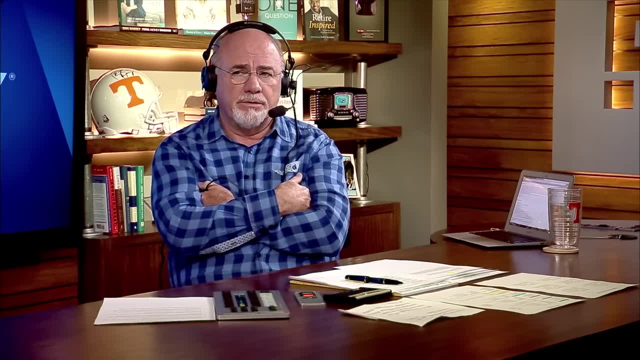 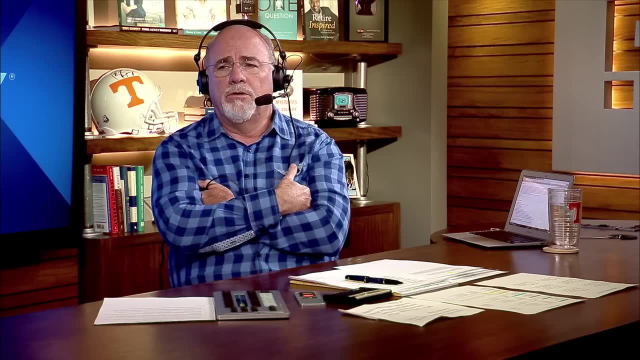 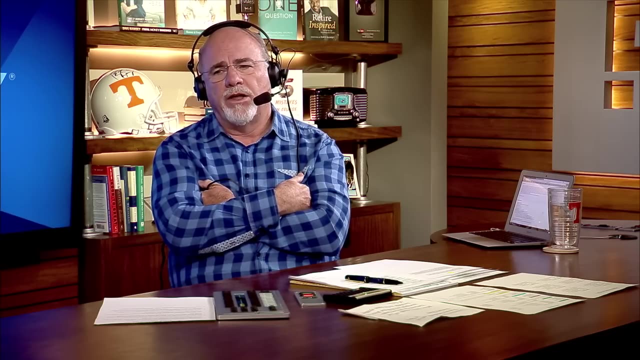 And you don't have a reliable vehicle. You've been doing beaters And so you know you need to go buy the car. You already knew that You weren't asking about that, but you already knew that. But maybe also take a little bit of that money and give it. Find some place to be generous. 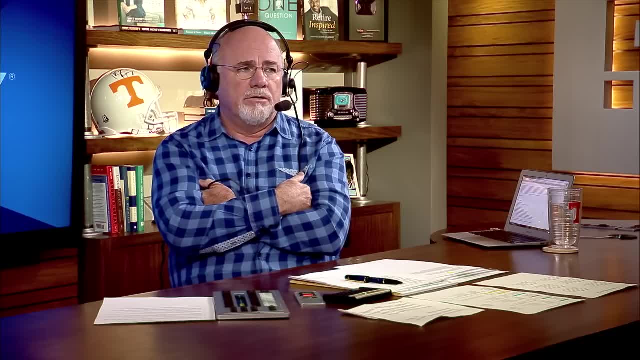 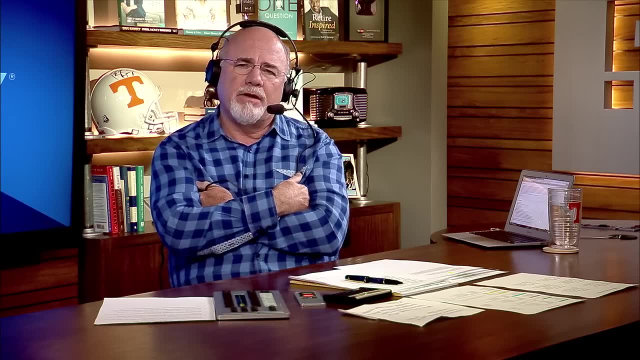 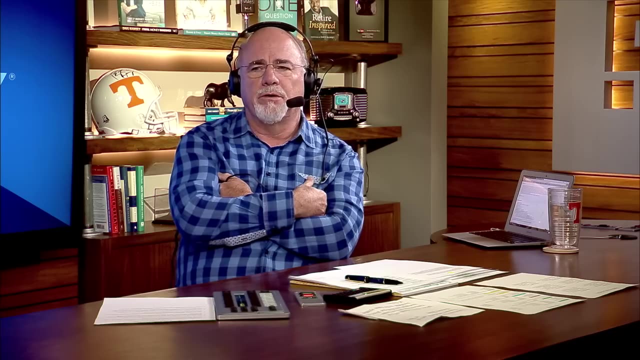 at your church or find a couple that's struggling or a single mom, Then pay her light bill for a year or whatever, But find something to do, Because there's something about giving that kind of then gives you permission down inside your spirit to also enjoy. 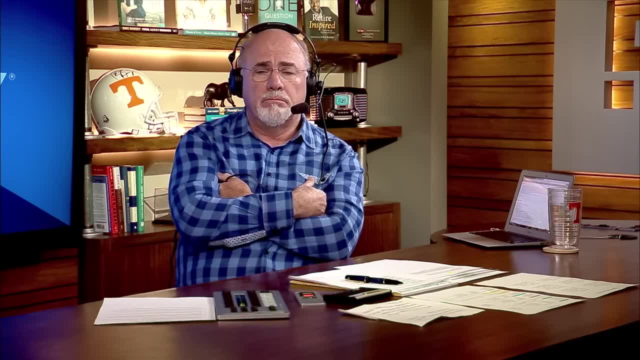 money, Because money's fun. if you got some, You ought to enjoy it. You ought to enjoy some nice things. Now, if that's all you do and you don't save and you don't give, then you're just a shallow twerp, right? But you know to assume that just because someone has 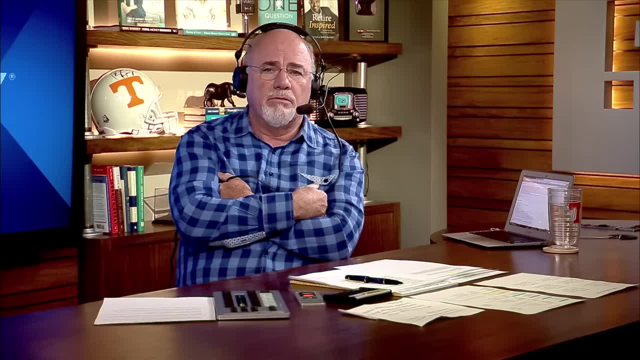 the ability to enjoy money means that they're greedy or shallow. that's just bogus, And the way you can tell is what percentage of their financial situation is going towards stuff for them. And if all the money you make is going to buy you crap, then you're out of balance. 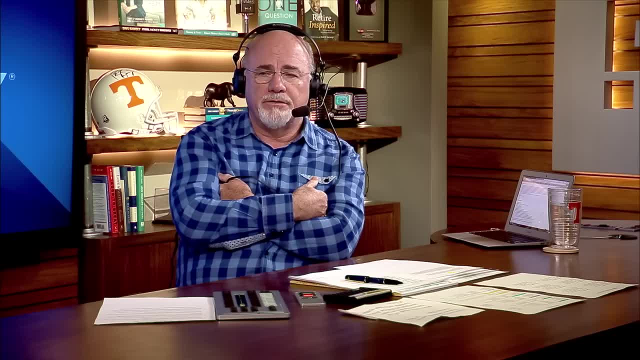 you know. But if you're giving a percentage of your income and you're investing a good percentage of your income, then you're out of balance. And if you're giving a percentage of your income and you're investing a good percentage of your income, then you're out of balance. 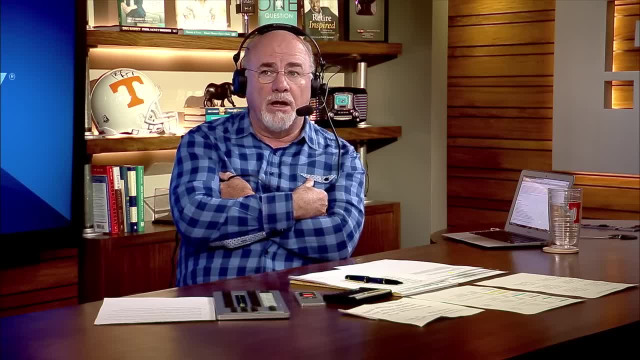 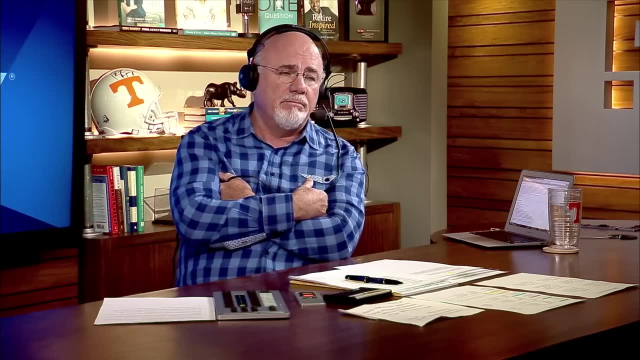 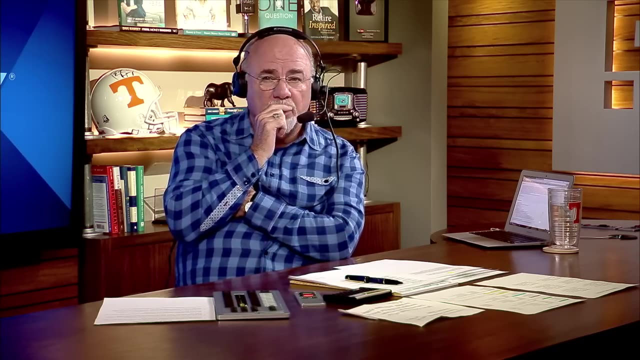 And if you're giving a percentage of your income and you're enjoying some of your income on lifestyle purchases, travel, cars, clothes, whatever it is- then that's in balance once you're at baby step three and beyond. And that's where Ricky is, But it's a really good question. 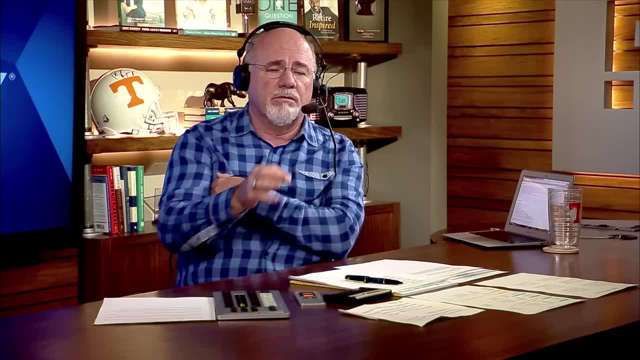 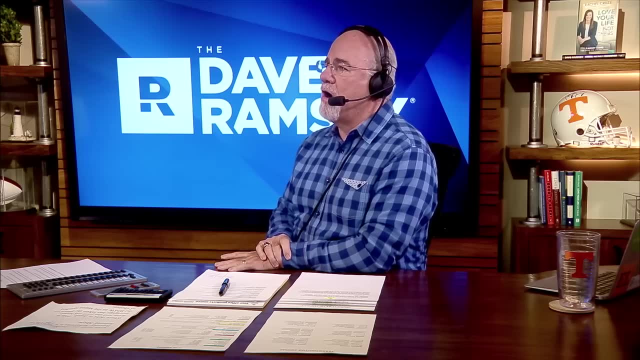 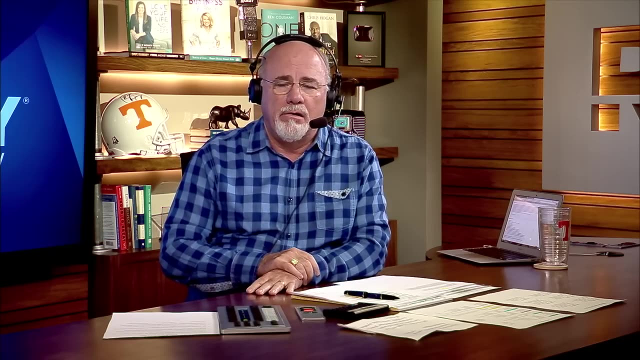 Ricky, It's a good question for me to stop and just kind of rant on or vent on for a second here. teach on for a second, Because sometimes people think, well, you know, no one should ever have a car like that. What would anyone need a house like that for? Now I've got a friend, that's. 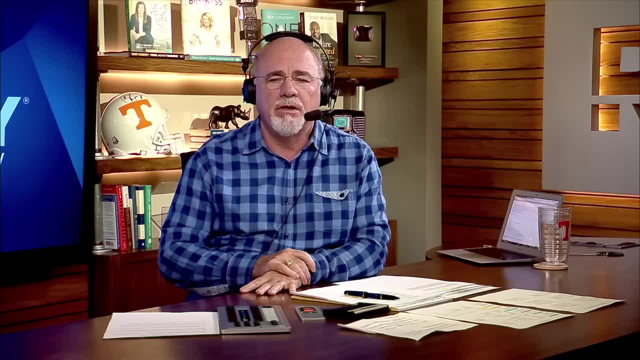 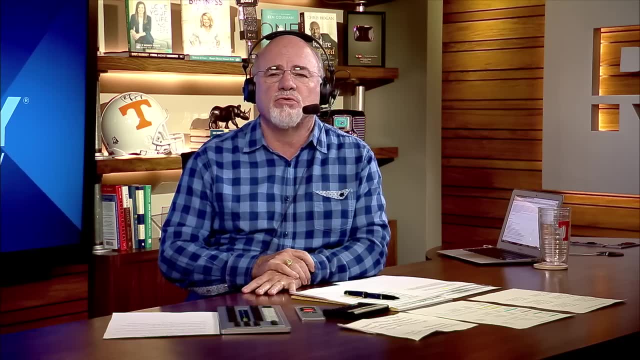 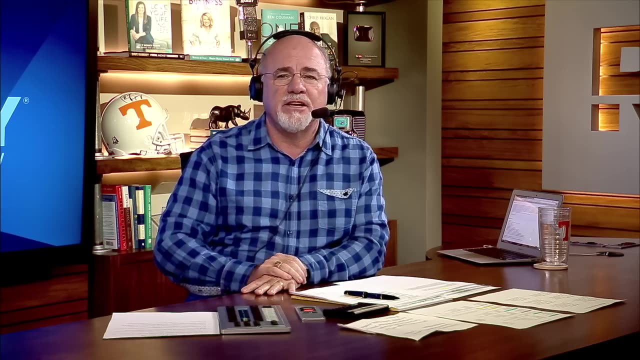 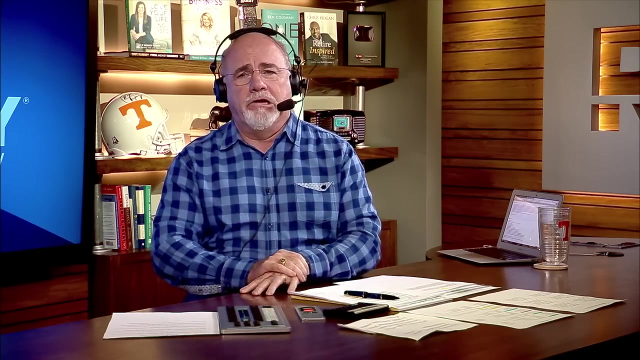 worth about three billion dollars. Now a billion is a thousand million. He has three thousand million. He has three thousand million. He spent six million on his house And people send him hate mail. No, I should ever have a house like that. His house as a percentage. of his net worth and his income is like you going through the drive through at Chick-fil-A and buying a biscuit. It didn't affect his life one iota to spend six million dollars on a house. As a matter of fact, that's a very conservative house for someone who has three billion dollars.